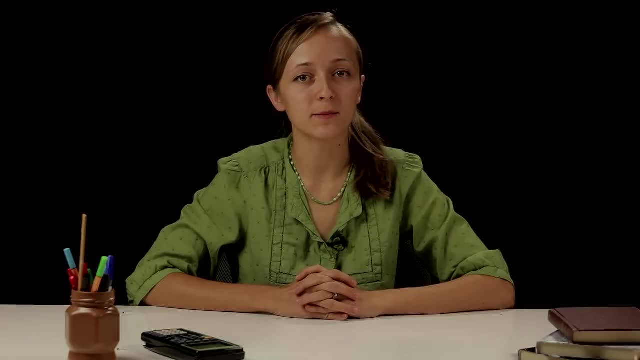 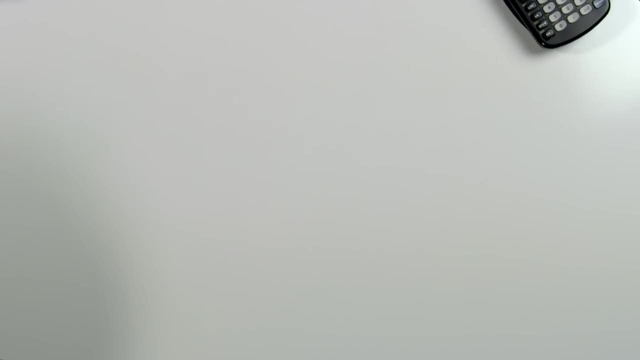 will happen. For example, suppose that we want to find out the probability of first drawing a green marble and then a blue marble out of a bag of marbles. We can write the multiplication rule like this: The probability of A and B happening, and here we use the. 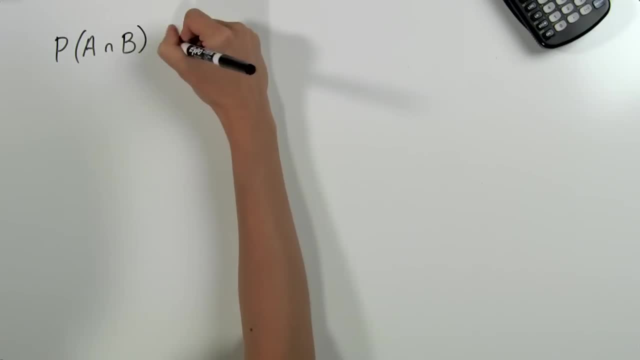 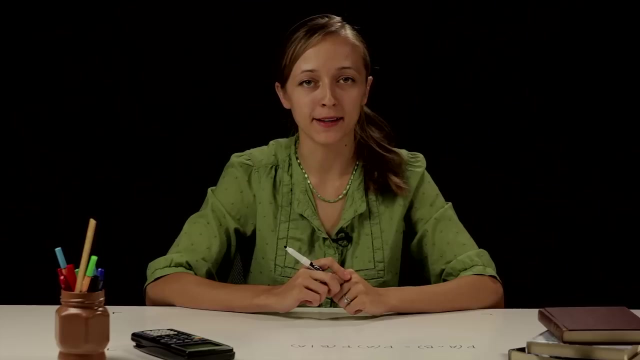 intersect symbol for A and B is equal to the probability of A happening times the probability of B happening, given that A has already happened. So let's go back to our example of a green and blue marble being pulled out of a bag. Let's say that there are 12 marbles total. 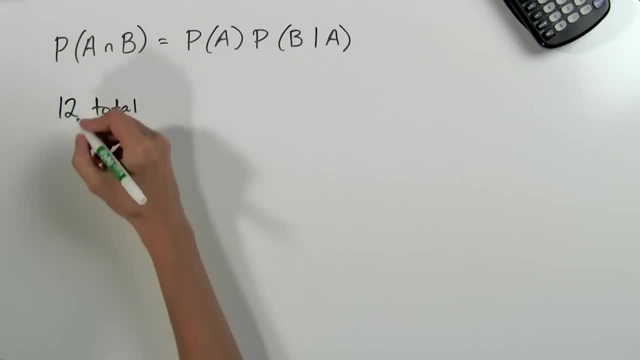 3 are green, 4 are blue and 5 are red. Our equation will look like this: The probability of pulling out a green and a blue marble is equal to the probability of pulling out a green marble. times the probability of pulling out a blue marble equals the probability. 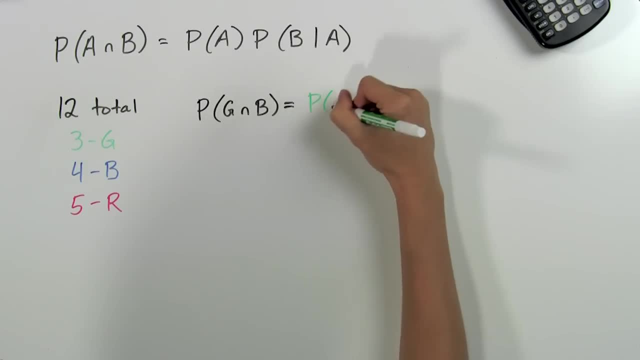 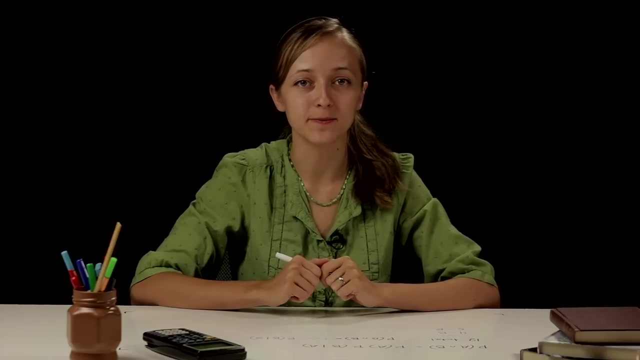 of pulling out a green marble times the probability of pulling out a difference in the length of the heard count of pulling out a blue marble after we've already pulled out the green. Now we just need to figure out what those two probabilities are and we can find the answer. Let's start with the probability. 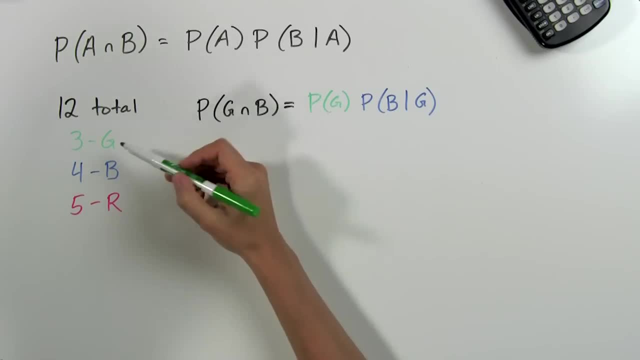 of pulling that first green marble. If there are three green marbles and 12 of them total, then the probability of pulling out one green marble is 3 divided by 12, which can be simplified down to 1 divided by 4.. Next, let's find the probability of pulling out a blue marble after. 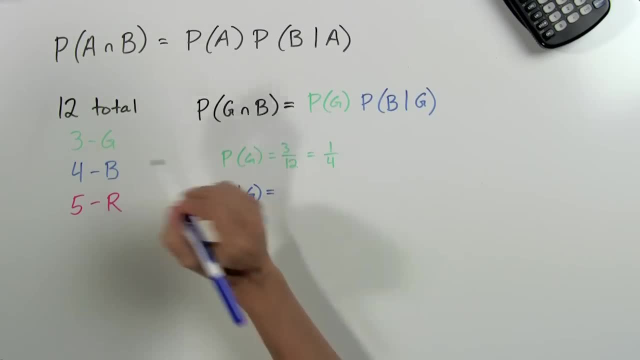 the green one. There are four blue marbles, so we can go ahead and write that in, but notice that we still haven't put in that first marble we pulled out. so now there are only 11 total. So we have four 11ths here. Now to get our answer, we can go ahead and multiply our two probabilities. 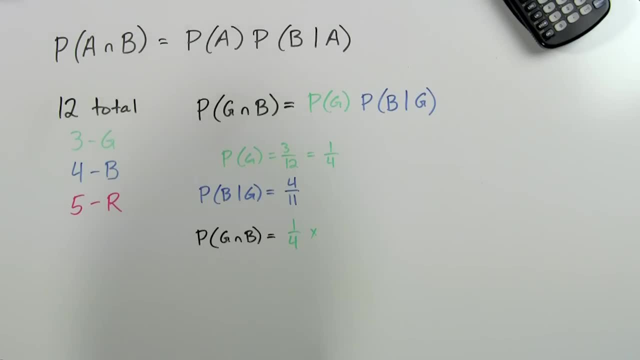 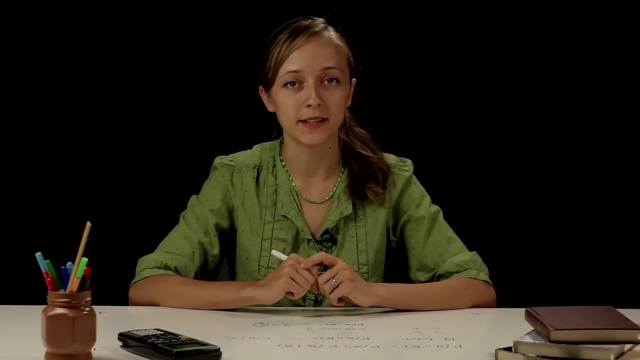 We have one-fourth times four-elevenths. The fours cancel out and we're left with one-eleventh Because we left the first marble out of the bag. this is an example of two dependent events. That means that the first event